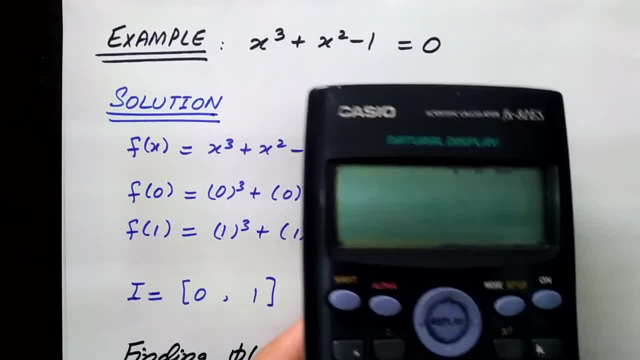 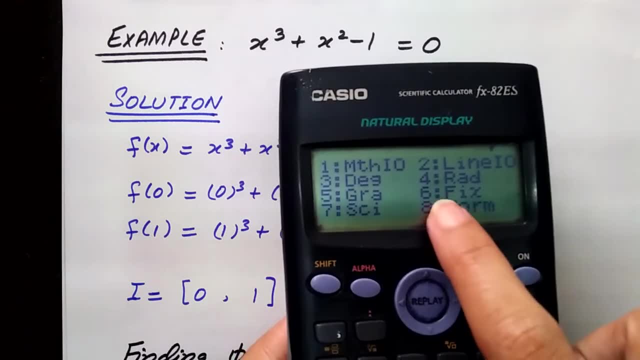 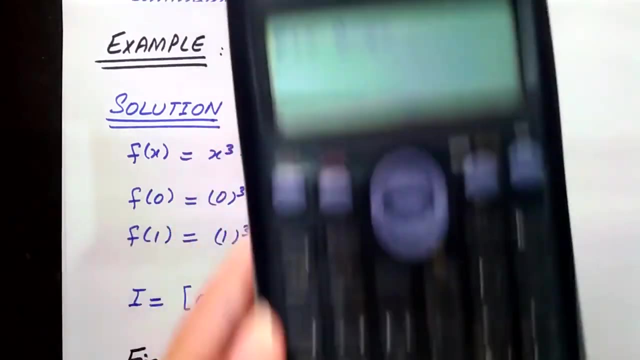 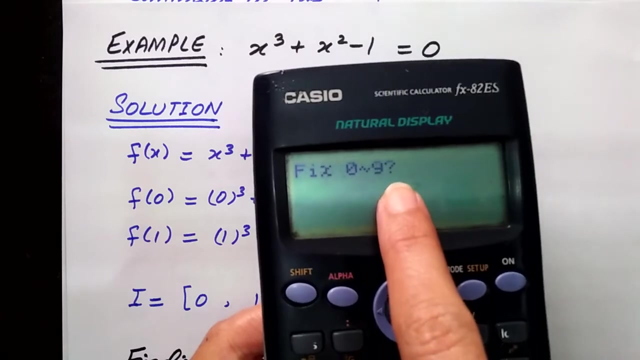 just press x1.. shift and then this mode. the point six is giving the function fix. so I will click six from here I will get the options: how up to how many decimal places I want to fix my calculator. I want to fix up to five decimal places. so 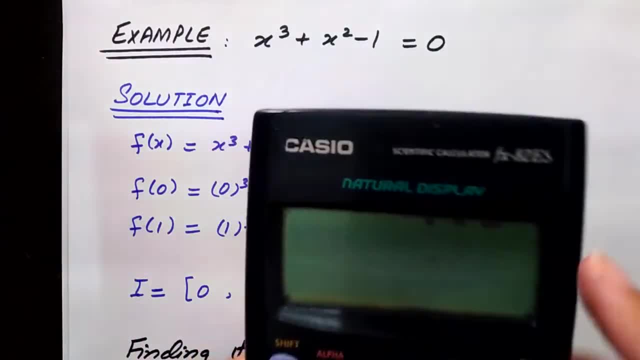 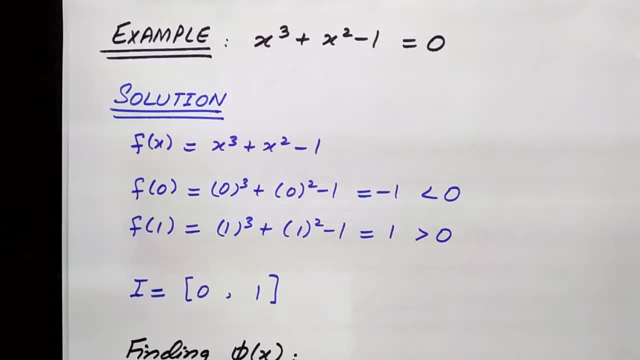 I will click five from here. so my calculator is now fixed up to five decimal places. x cube plus x squared minus one is basically f of X. now I want to find out an interval on which this function f of X is showing different behavior. I checked for zero and one put zero in. 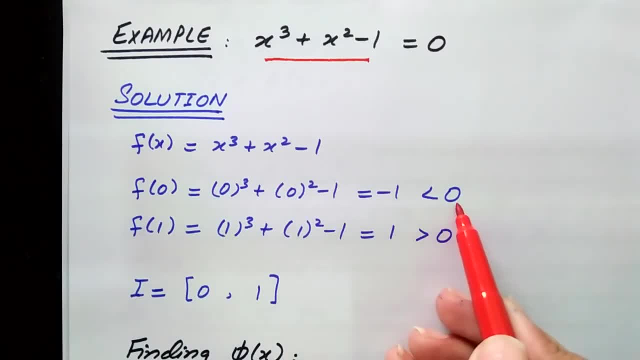 the 10 egg in the box and then follow the same procedure. next, now I have a еюсь 0 and 1, put zero in the 1000 and hit enter and go. get less than root 0 and function. the function shows the negative behavior and when i used value of x equals to 1. the 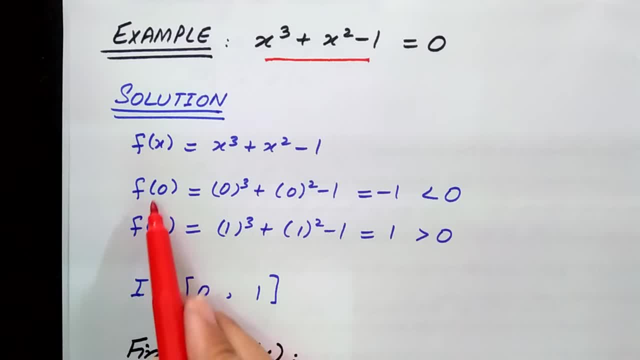 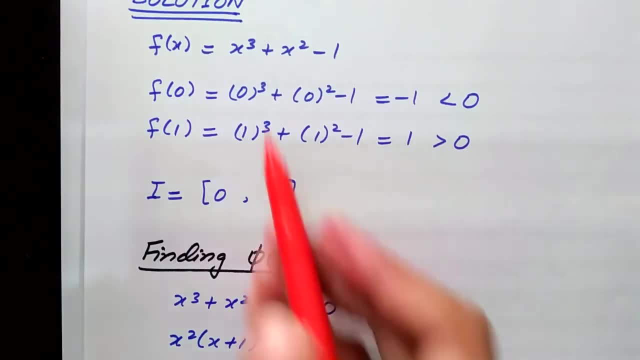 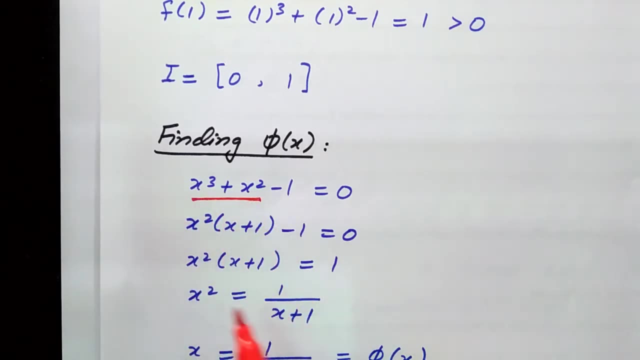 function showed the positive behavior. this means my root lies between 0 and 1, so the interval will be from 0 to 1. now for finding phi of x. consider this: f of x equals to 0. i took x square common from the first two values. my equation reduced to x square into x plus 1 minus 1. move this minus 1. 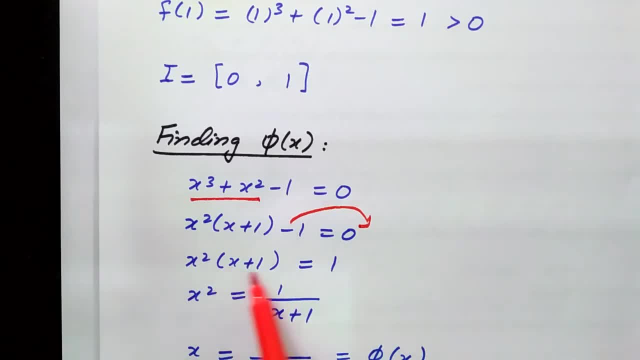 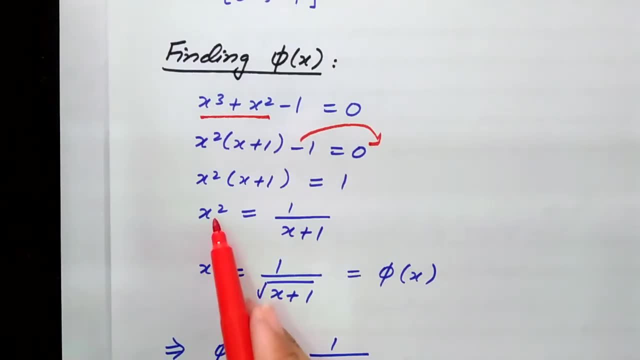 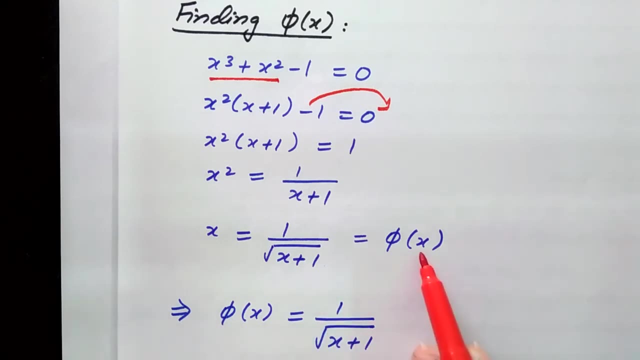 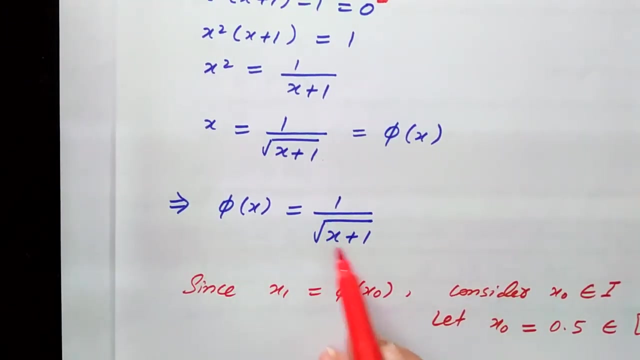 on the right side the equation took the form: x square into x plus 1 equals to 1. so x square equals to 1 over x plus 1, and for removing this square i will apply square root on both sides. so i got x equals to 1 over x plus 1, that is, equals to phi of x. now a phi of x equals 1 over under. 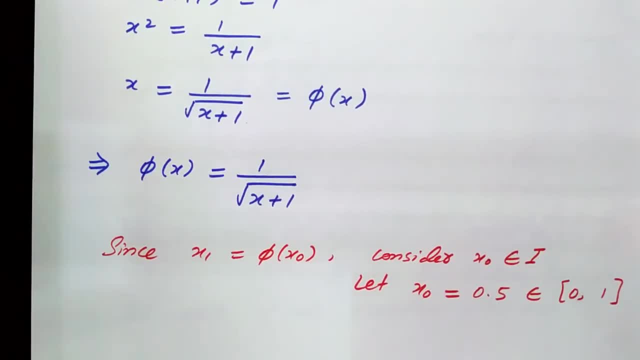 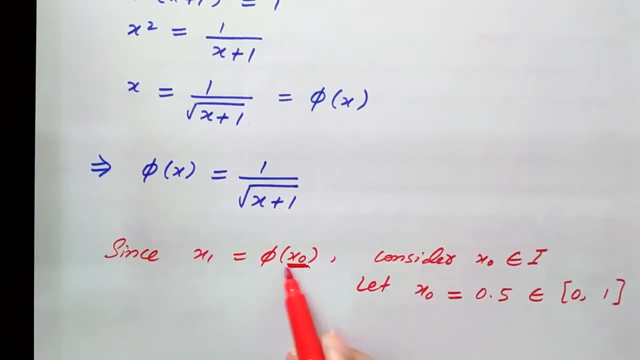 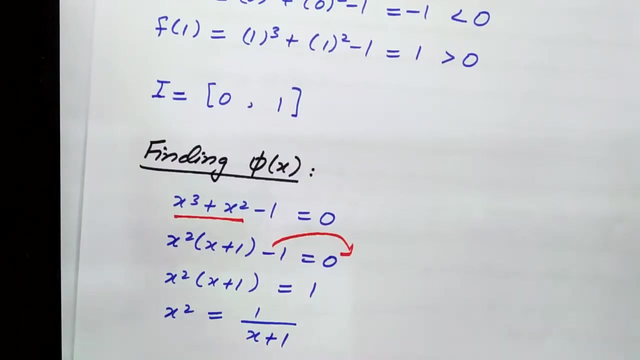 root x plus 1, since the first value, that is x1, can be obtained by phi of x naught. now question arises here that what is this x naught? i will consider this x naught from my interval that i took earlier. my interval is from: 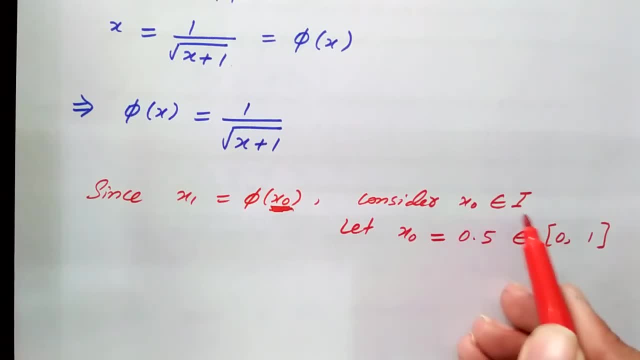 0 to 1, so i will consider any value from this interval that will be equals to x naught, for example. i considered here x naught equals to 0.5. this 0.5 is basically from 0 to 1 the value. 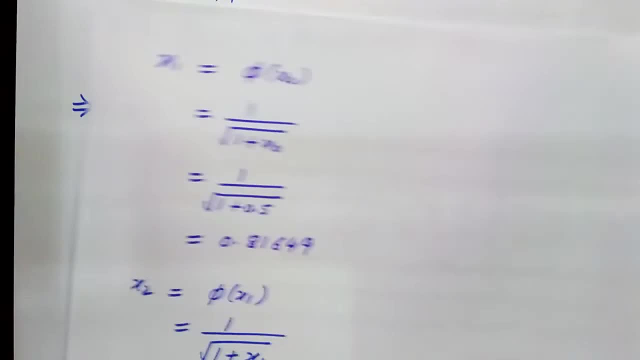 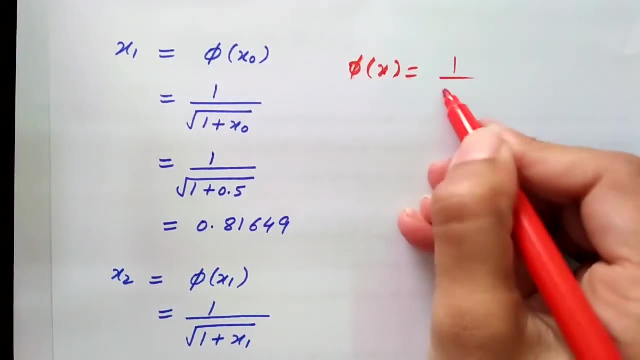 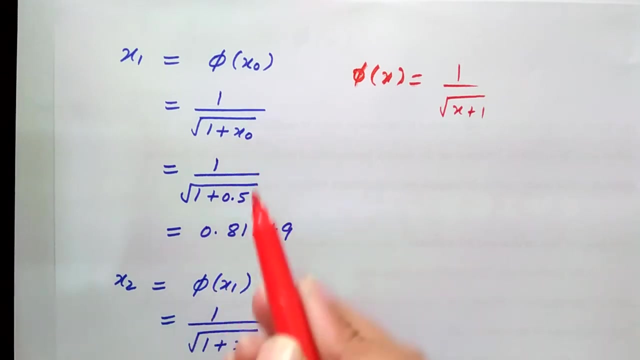 between 0 and 1. x1 equals 5 of x naught. my Phi of X was 1 over under root x plus 1. so in place of x i will get x naught. put the value of x naught. x naught I consider 0.5, so use the value of x naught. 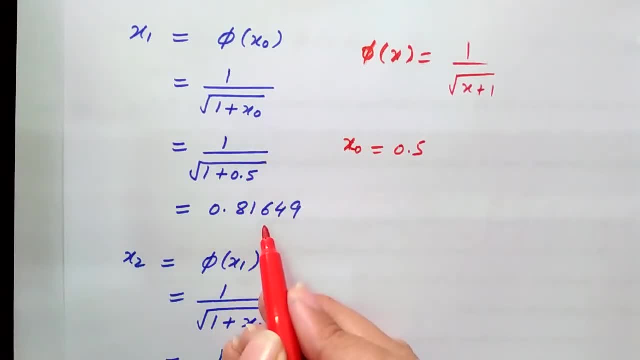 over here and simplify it using your calculator, you will get the answer of x: 1 up to 5 decimal 1. then you will get 1. beat吧 face- narration: n Voix feed en x1: 0 amount of f0. over here and simplify it: under root x plus 1. if x0 put into x1, we get a value of xn capital x: 0, and simply use the following Chinese calculator to get the correct answer: up to 5 decimal. place нач quality: 0.5. so here is the formula for f of x0 and also you can actually god2 quantity one zero decimal time value x0 is considered, but this is called as c Down rho. few points here. the test section only i left as db, right. so if this is the exact, 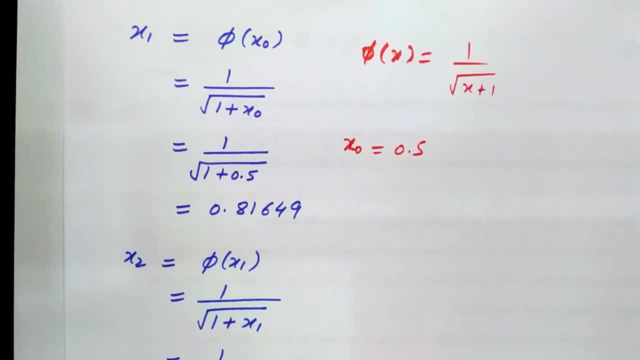 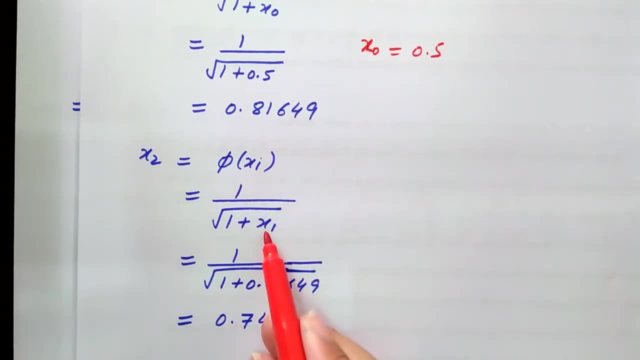 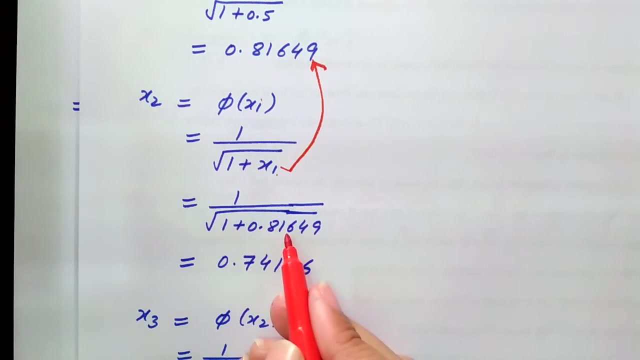 that I fixed earlier on my calculator. Then calculate x2. that is equals to phi of x1. I will use in place of X the value of x1 that I calculated here. This is the value of x1.. Put this value in this equation and I will get the value. 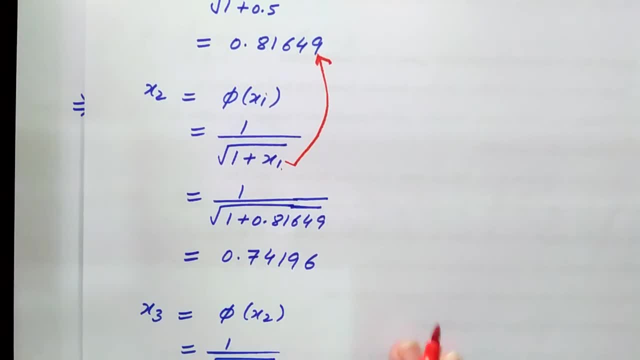 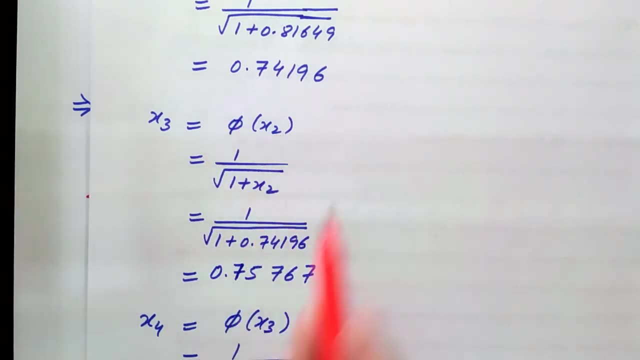 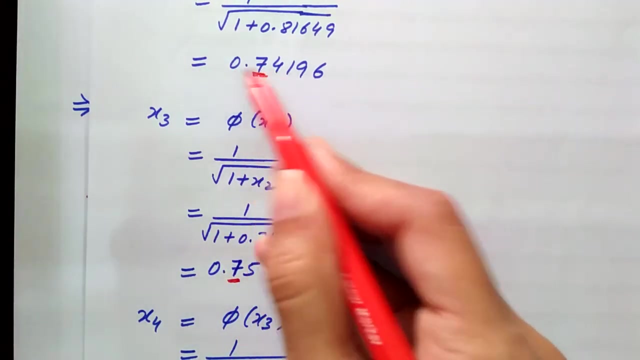 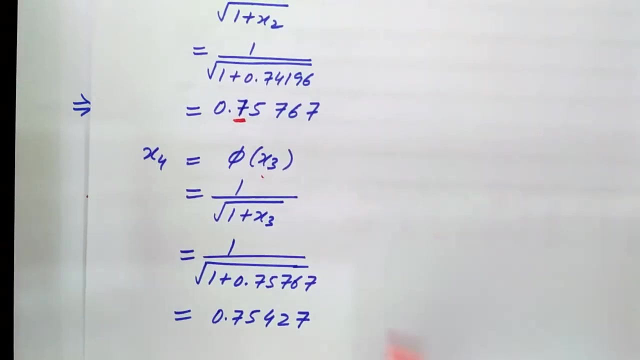 for x2.. I will continue my process until my root is repeated up to five decimal places. Now solve it for phi of x2.. I got 0.75.. See one up to one decimal places. my answer is repeated: 0.7, 0.7.. Now find the value for x4, that is, phi of x3.. I got 0.75.. 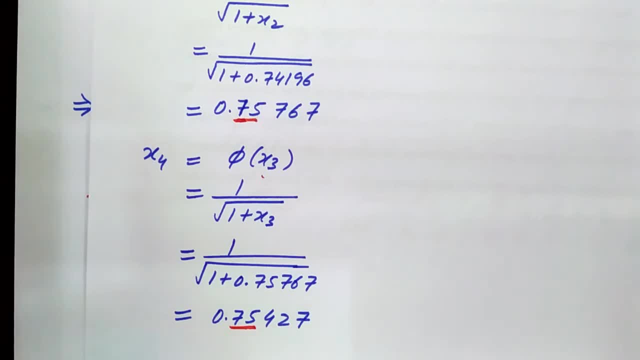 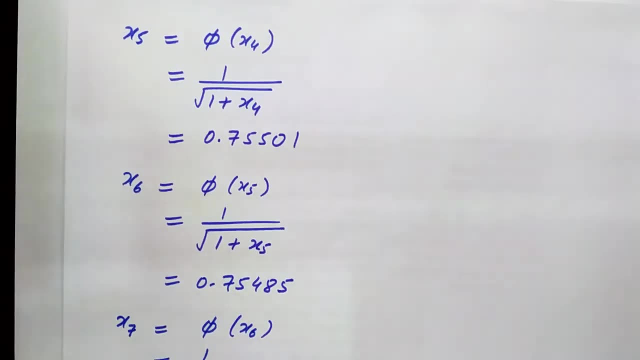 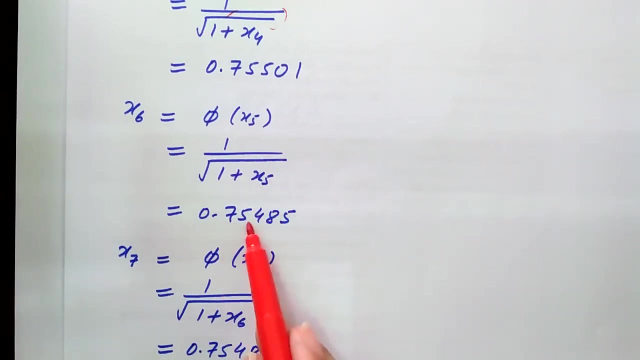 Up to two decimal places, this answer is repeated. I will continue this process until my answer is repeated up to five decimal places. you Now: x5 equals phi of x4. Use the value of x4 in place of this equation and I got 0.5501.. Then x6 phi of x5. Use the value of x5. I got 0.75485.